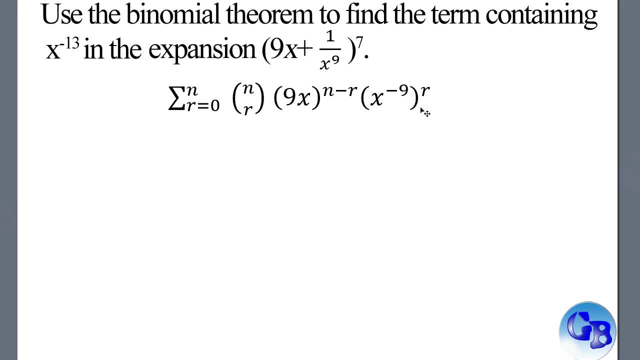 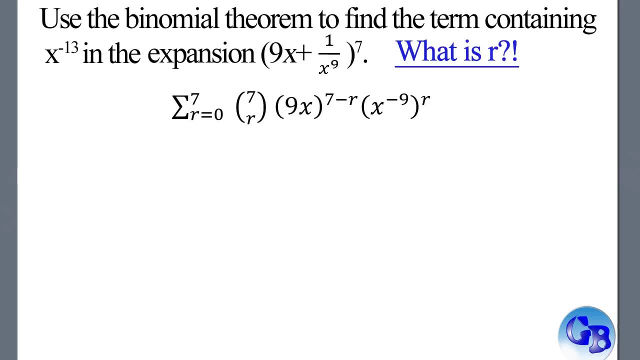 So what we want to do first is we'll plug in what numbers we do know. Well, we do know that we are dealing with it to the power of 7.. So that's going to be n. So when we plug that in here, we now have our binomial theorem: with 7, choose r, 9x to the power of 7 minus r times x to the power of negative 9, all to the power of r. 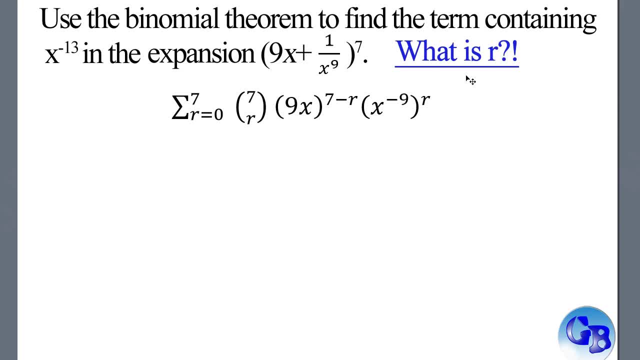 So our next question is: how do we solve this? We need to know what is r. So what we're going to do is we're going to come down here, Let me grab my pen tool and we are going to just write. 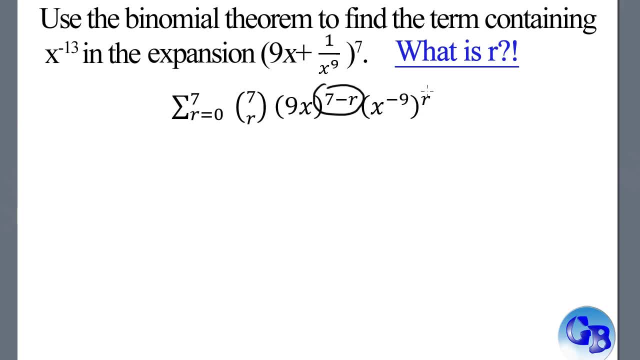 We're going to write out our exponents here and we're going to start solving for r using those exponents. So we have 7 minus r and then it's going to be negative 9r because we just brought those two together. 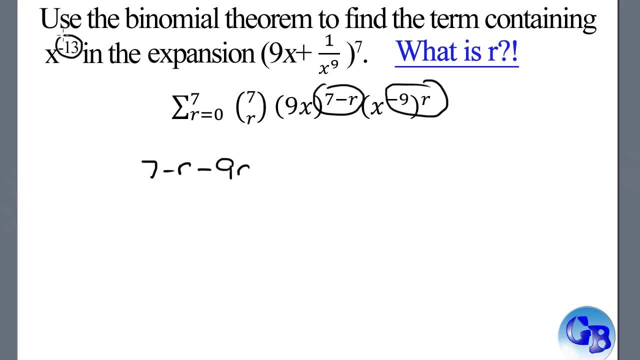 And since we know that we do want to get to x, to the negative 13,, we're just going to set this equal to negative 13.. And from there it's rather simple We can solve. We can solve for r by basically doing our simple basic algebra: negative 10r equals. we're going to bring the 7 over here. 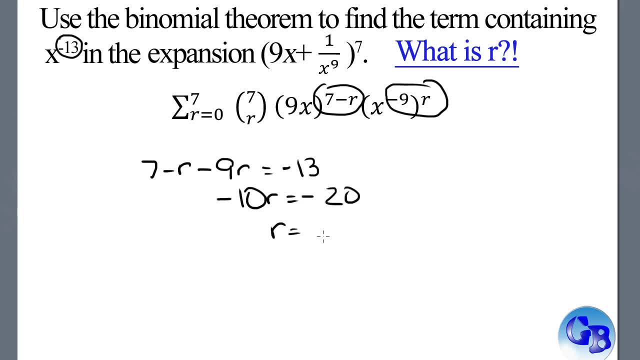 We have negative 20, and now r equals 2.. So now that we know that r equals 2,, all we have to do is simply do our plug in our numbers and see what we get. So what we're going to do is say 7, choose 2, and then we're going to multiply 9x. 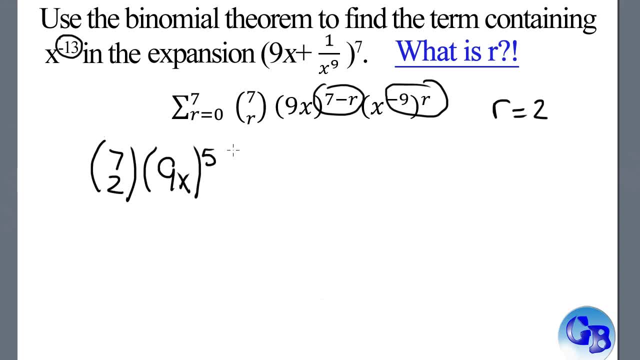 So we have 9x to the power of 5, because 7 minus 2 is 5.. And then we have x to the power of negative 18, because negative 9 times 2 is negative 18.. When we plug in our values, we get, for the first one, 21..